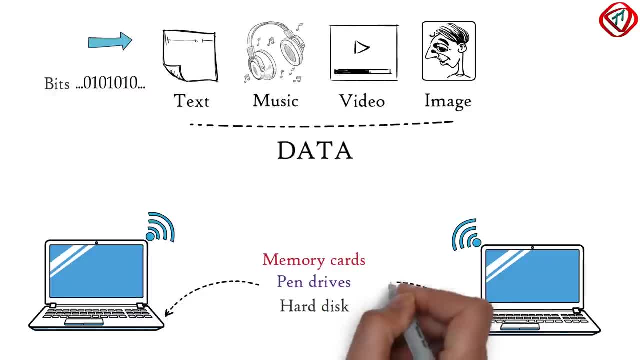 So when we transfer a file from a pen drive to a computer's hard disk, we move and store a sequence of binary bits. CPU process these bits and present them. We send a text file on the computer's screen which we can read. 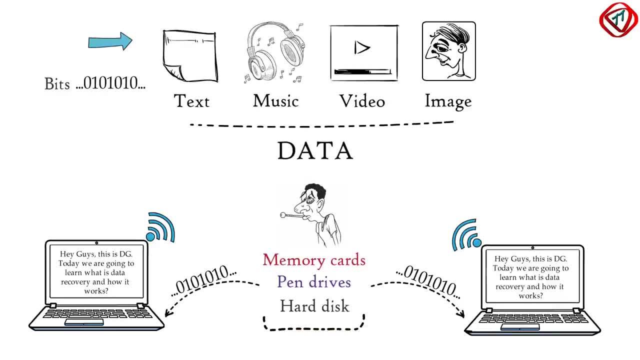 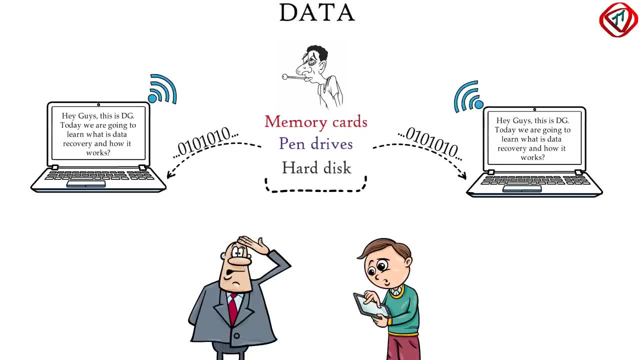 However, there are chances of getting these storage devices corrupted, which can lead to loss of essential data, And we too can accidentally delete some critical files from our devices. In such cases, is there any possibility of recovering the lost data? The answer is yes, we can recover it. 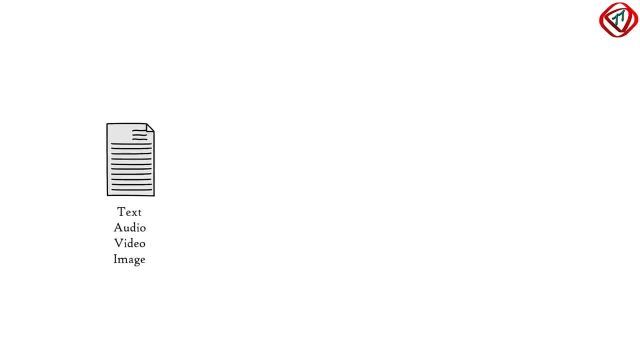 And the process is called data recovery. Each file present on a storage device has a pointer which tells the operating system where the file's data start and where it ends. As long as a file has a pointer, it can be seen on the computer's screen. 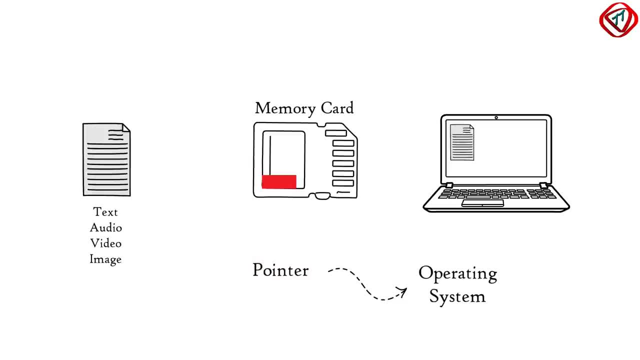 However, when this pointer is no longer available, the operating system cannot blockade the file and takes it to be deleted. The same thing happens when you delete a file from a computer. The operating system deletes the pointer of the file and marks the space it occupies as unreserved. 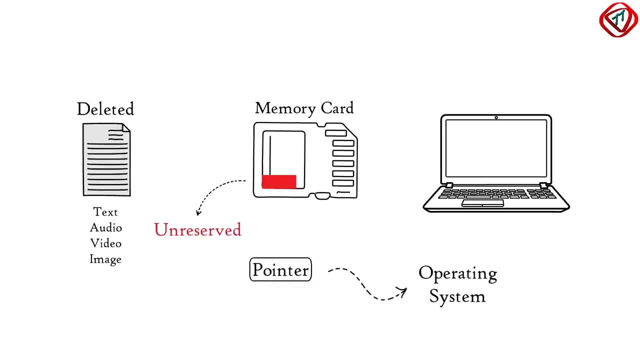 Since deletion only deletes the pointer and not the actual file, the deleted file can be found and recovered from the storage device. until or unless any other file overrides the deleted file's space, The only need is to regain the pointers. There are many tools available in the market which performs the same function. 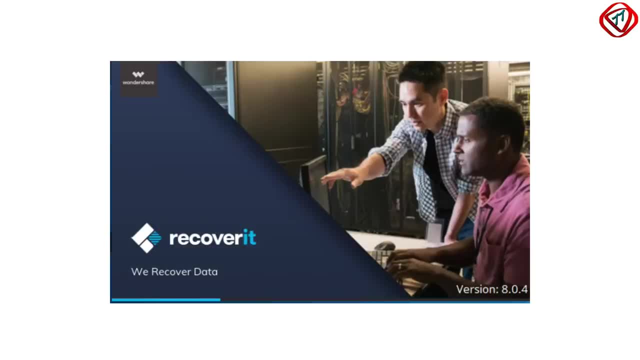 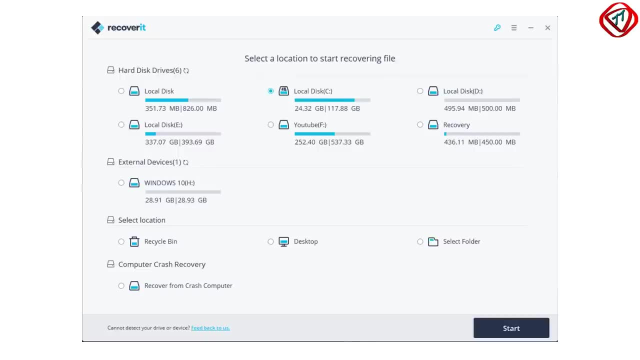 One of them is Recoverit, which is also the sponsor of this video. Recoverit 8.0 comes with a simple user manual. It has a simple user interface and provides us the option to recover data from any drive within the computer's hard disk. 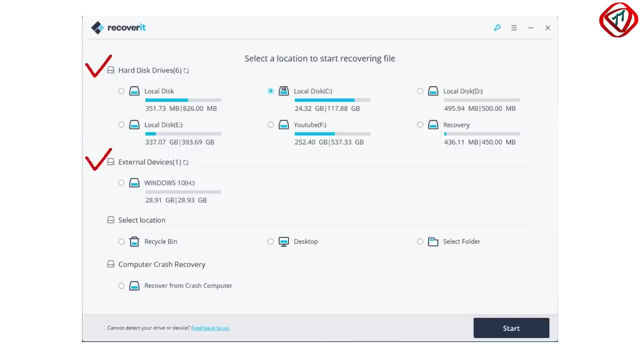 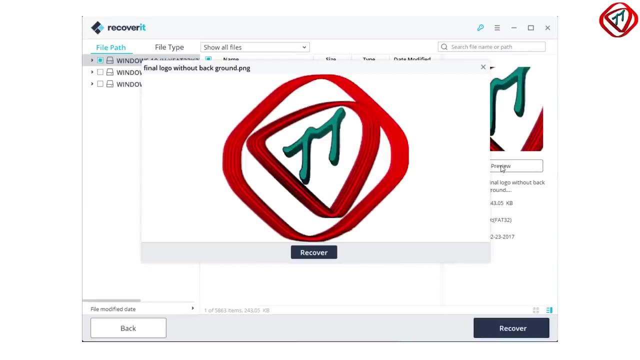 It can also recover data from externally connected devices and even supports computer crash recovery With Recoverit 8.0,. a particular location can also be selected for data recovery. Once the lost data is displayed, we can preview it before recovering it. Right now, Wondershare is offering free 1-month promotion.